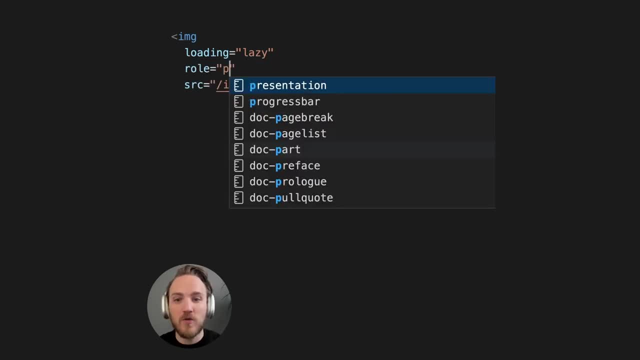 accessibility, Or if this image is presentation only, use role equals presentation, to be a bit more equivalent to like a CSS background image. Next is the ability to control an entire source sets, And this is a more powerful version than you get with CSS, Because with this, 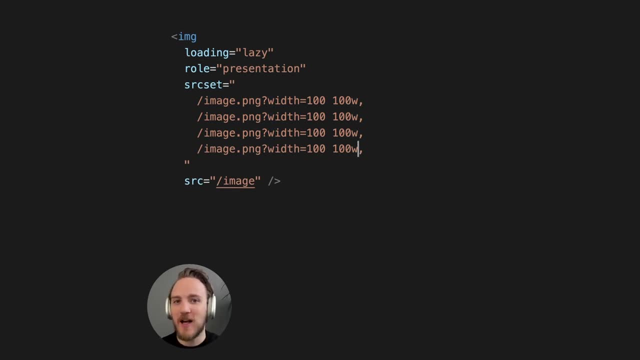 we can use the W unit, which automatically takes into account both screen size and screen resolution. So an image currently displaying to a user at 100 pixels wide but at 2x resolution will grab the 200 wide image or the closest variant you've provided, And the browser does. 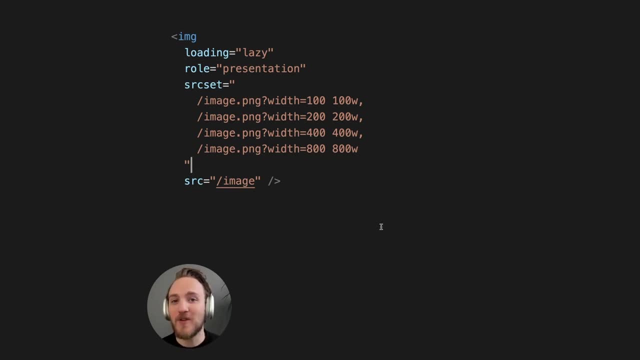 this completely automatically. Now that does require, though, the browser to have rendered the image to know the size, to pick the most optimal version. Otherwise, it could default to an image that's too large. That's where we, additionally, get the sizes attribute, where we can say at: 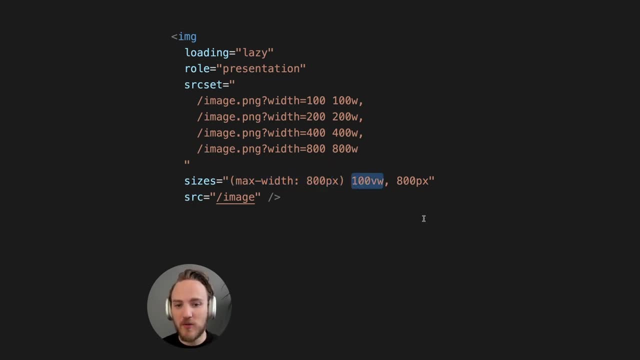 different screen sizes what the relative width of this image will be. So maybe it's 100% of the view width at this size And for the rest maybe it's half of the view width. Now the browser, even before the page renders, can pull the most optimal image. One more major optimization we can do here: 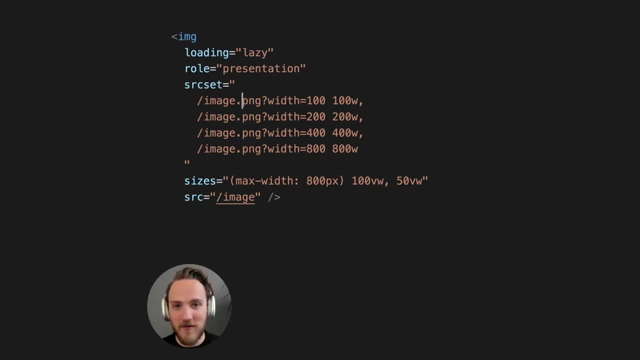 is to recognize we're using PNGs. These are supported by every browser, but not the most optimal. in most cases, This is where we can add the picture tag around our image, And now we can use a source tag specifying a WebP version of this image with its full source set. So now every 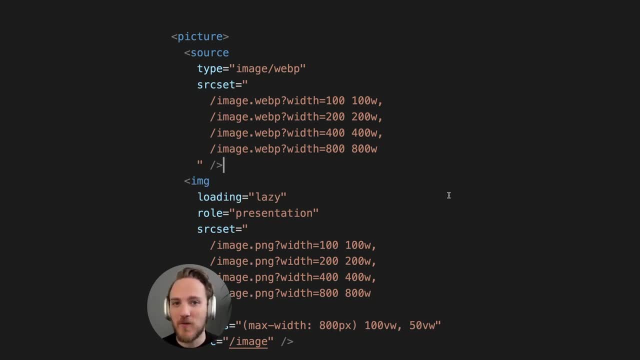 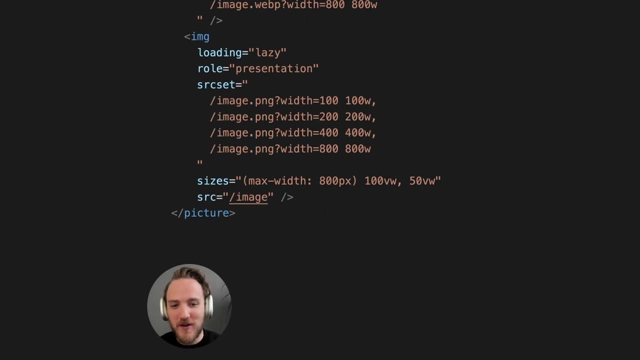 browser that supports WebP will get a faster loading image with all the same optimizations. We can even do the same thing with other formats, like AVIF, if we like as well, And if we want to take things even further, we can specify what type of decoding to use, like async. 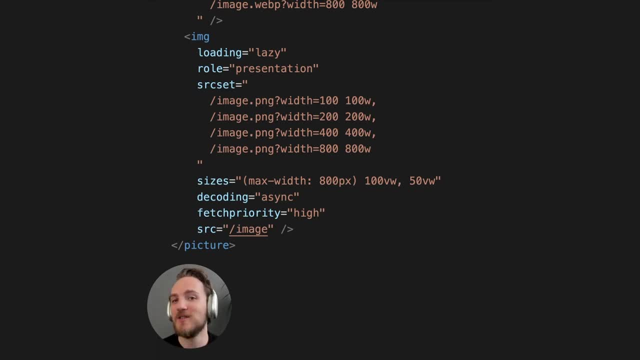 as well as the fetch priority of this image. So there's a lot you can do to ensure your images load as fast as possible, which can make a big difference for your site performance. But if this seems complex, you're in luck: Modern frameworks like Nextjs and Quick. 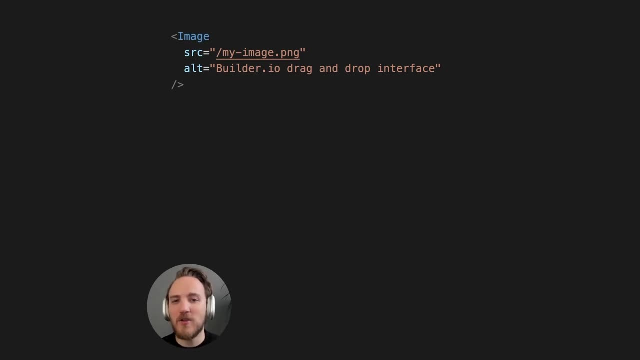 provide you with easy to use image components out of the box. So you just apply the path to the original image And most, if not all, of those optimizations are done for you automatically. And if you do or don't use one of those frameworks- more and more services these days-